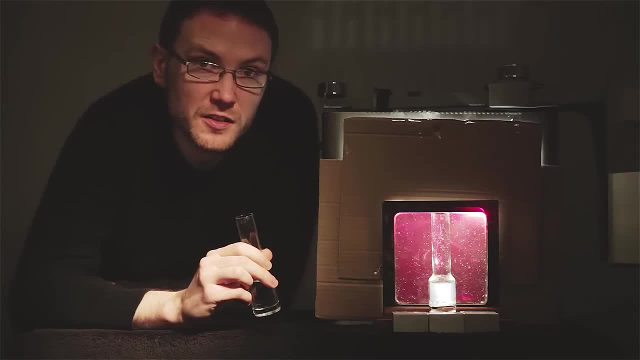 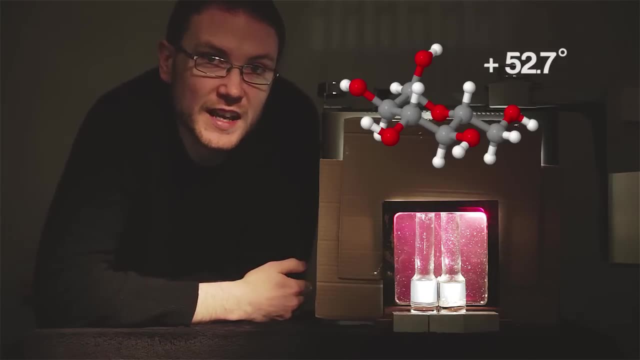 Other sugars, like glucose and fructose, are chiral too. Glucose rotates lights to the right, hence also being known as dextrose Fructose, which is sold in supermarkets as fruit sugar, rotates lights strongly to the left and is also lesser. 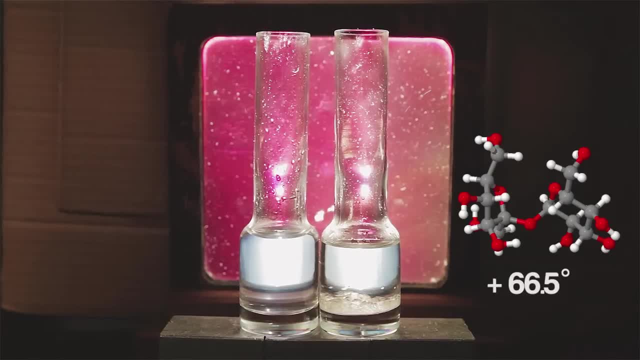 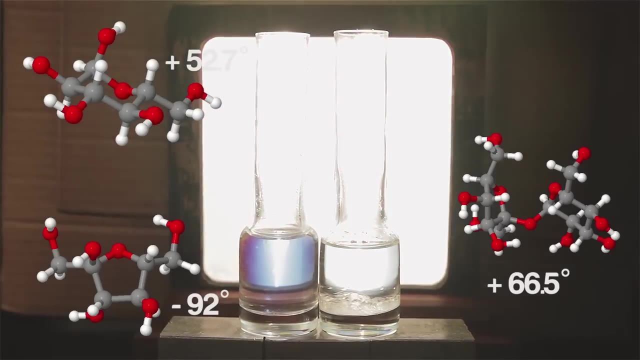 known as levylose. But have I just added a glucose solution or a fructose solution? Both look the same. I don't think so. However, if you turn one of the filters back and forth, you can see our solutions are rotating in opposite directions. The one on your left is fructose. 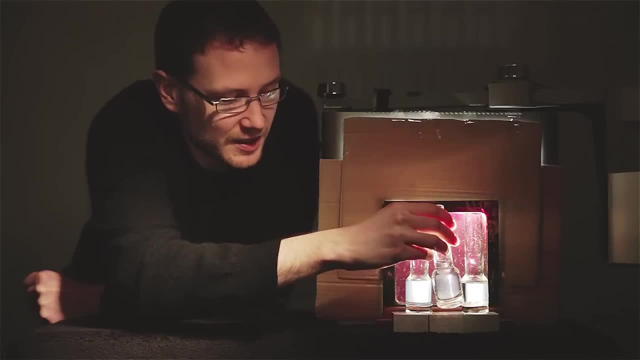 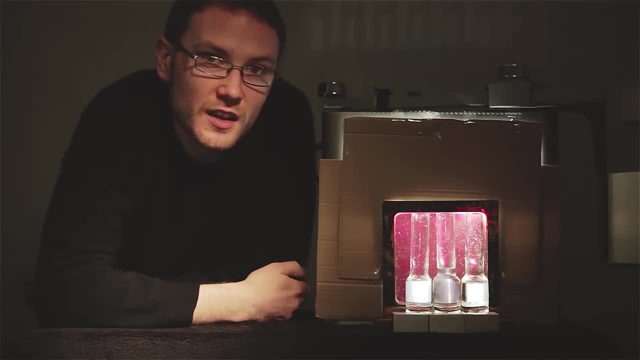 Now here's a cool extension. This solution here starts off exactly the same as the sucrose solution on your right. I added a few drops of lemon juice and then boiled gently for about five minutes. Sucrose is a disaccharide solution. It's a very simple solution, but it's also very 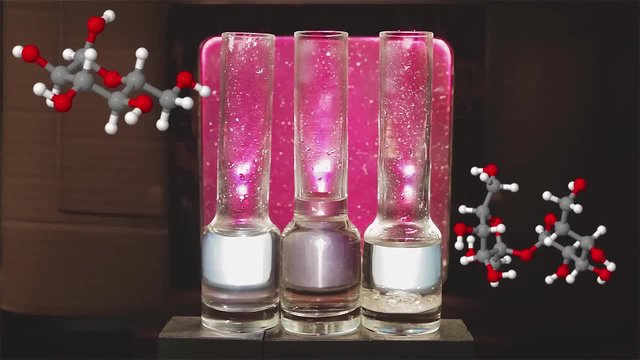 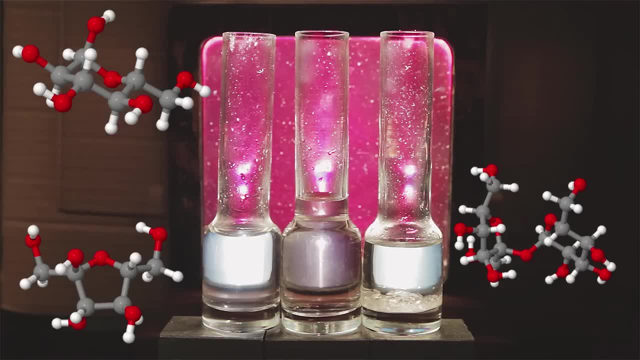 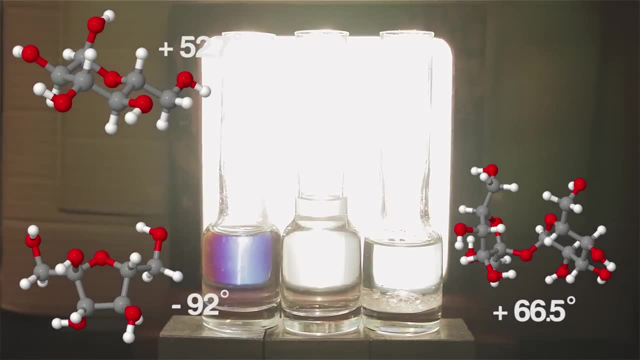 right. glucose rotating right and fructose which rotates strongly left. Watch as I rotate. The solution in the center now rotates somewhere between the other two Left. hydrolyzing long enough, the solution will begin to rotate left, hence being known as invert sugar syrup. 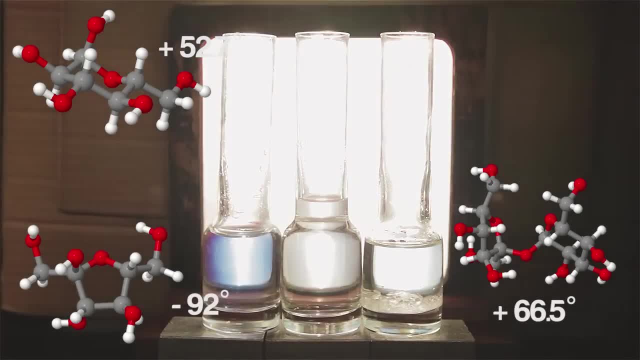 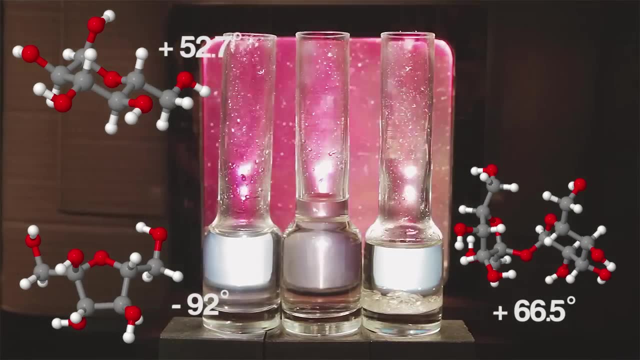 When the sugar sugar which is farms required for the social protection stage of glucose relationship with sugar, this solution is given its best credit. This planet's cell is fooled into thinking that something's going on and that its Deputy Previously at the Technical Institute of Academy of Science Motor yo rome성을 has recorded. 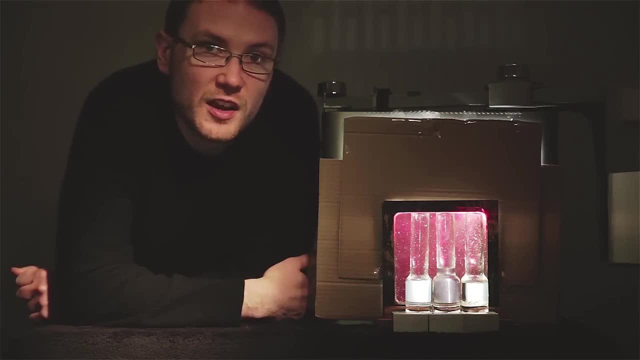 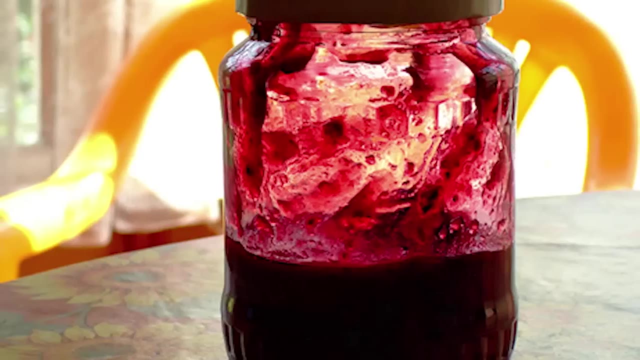 a story about what was happening in小心burgalt and what went on with the理学学. Invert sugar syrup is highly prized by the food industry because, compared to sucrose, it's sweeter, it has a lower water activity, which means it has a longer shelf life, and 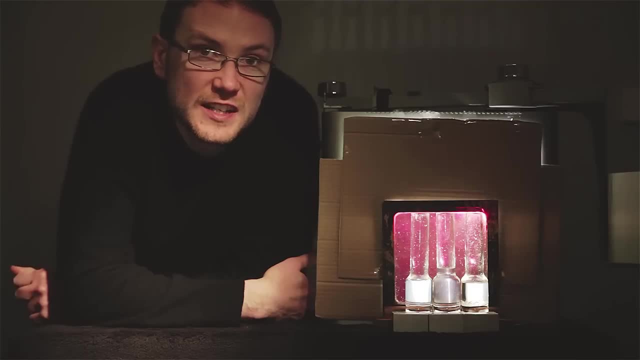 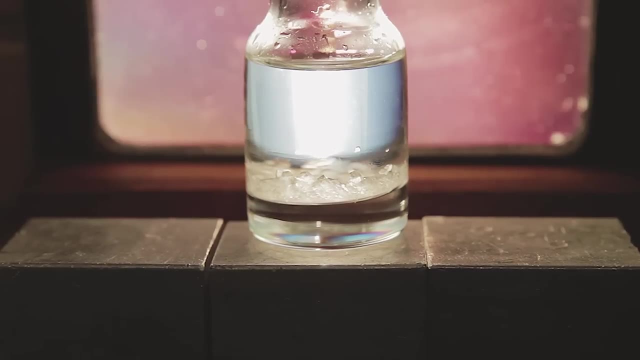 also, it's less prone to crystallisation. The reaction in industry is actually followed by polarimetry. I've had these flasks for a few weeks, so they'll keep long enough for a whole year group to see. You can, however, see that the sucrose has begun to crystallise, whilst the fructose and the